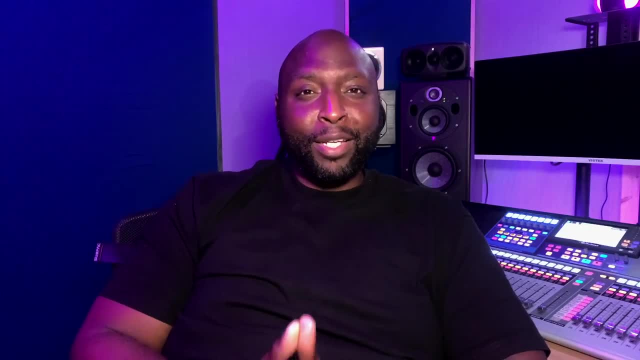 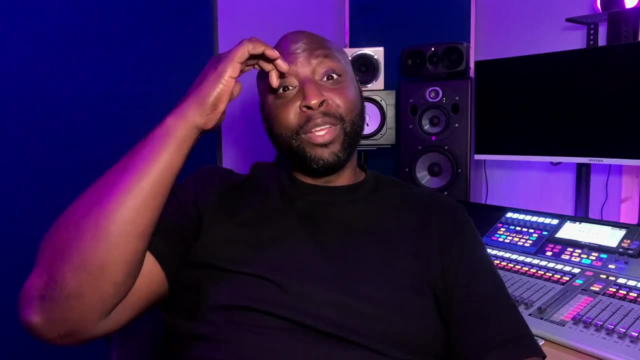 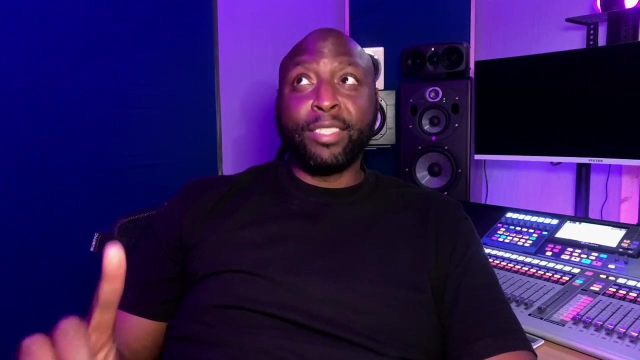 started piecing it together. that's exactly what I mean, so I didn't start. I definitely didn't start with the way the studio is now, with all these studio monitors and mixer boards and stuff like that. I started off with a two computer- actually was one computer that had two screens and 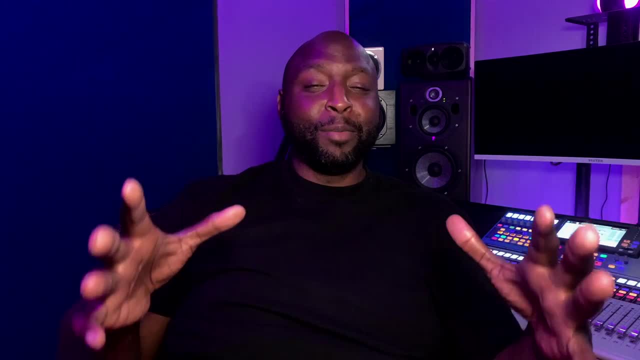 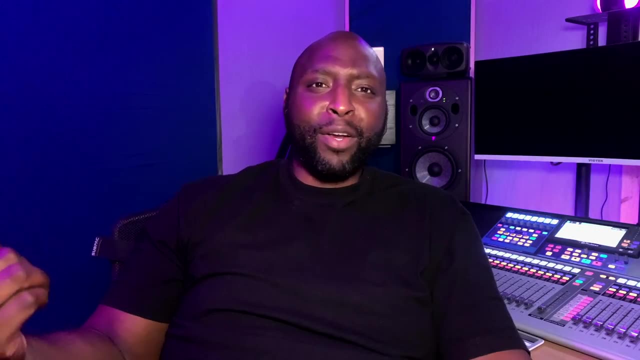 back then I, those were the big fat screens, you know I'm saying so, the screens with the big fat backs. I had two of them and I had them sitting on my desk and I bought a card for my, my computer, so I can have dual screen. I thought I was doing it, you know I'm saying, but the idea was I wanted to. 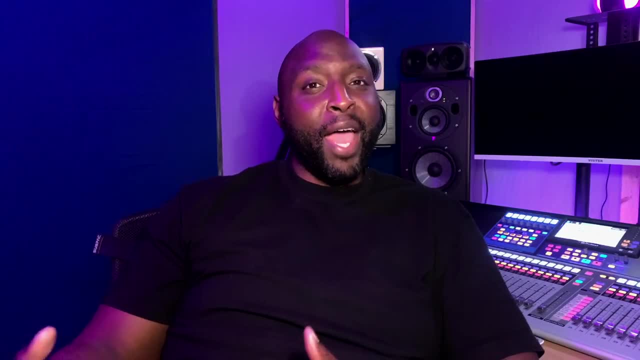 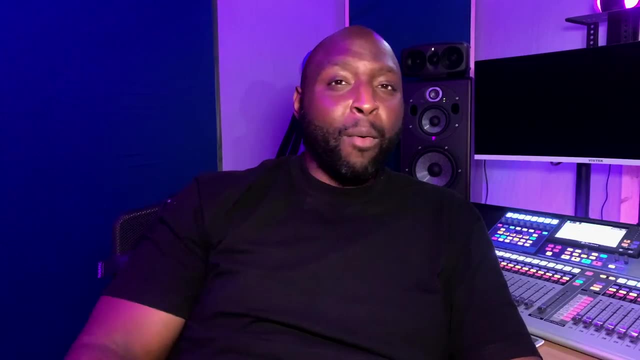 make sure that when I was working on my computer, I was working on my computer, I was working on my music. I actually had more time than when I was in the studio creating the music or relaying the music. so I would write the music at home and then I would go to the studio. then I just recite my 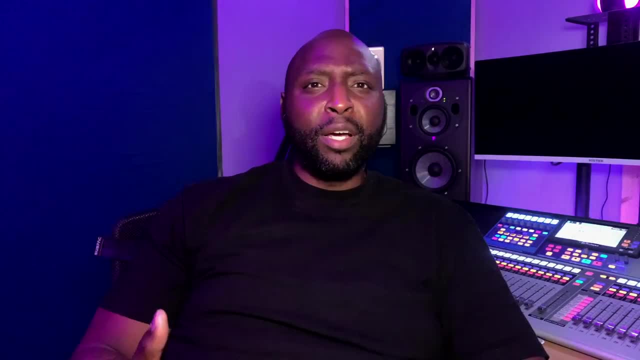 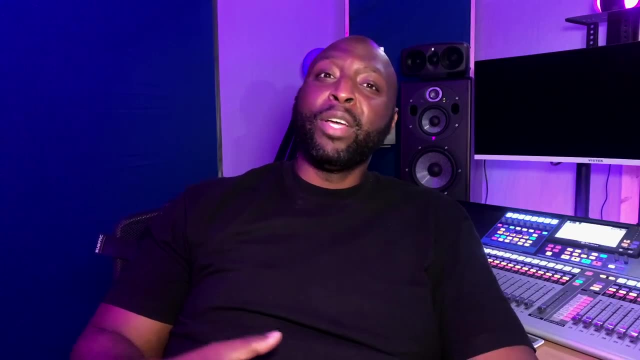 verse, but I always thought to myself, if I had more time in the studio, like what could I come up with? and you might be in this situation right now. so I'm just want to explain to you what audio engineering is, because there is a difference, and maybe you know it is something that you want to do, or maybe. 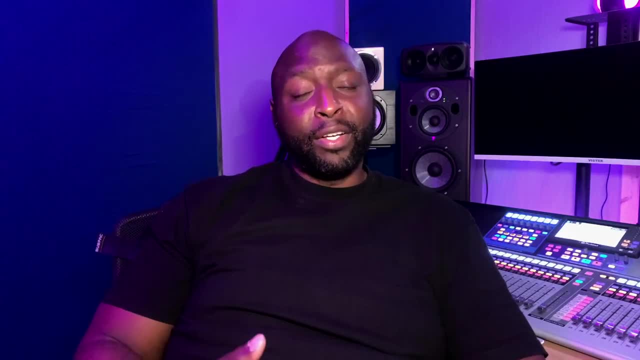 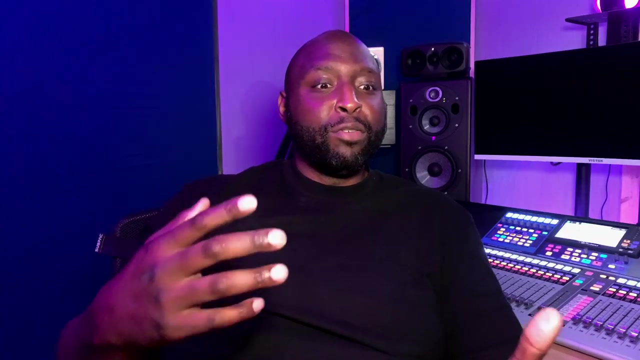 it's something that you just strictly don't want to do. the basics of audio engineering is manipulating sound. so basically, what you're going to be doing- if that's what you choose to do- is you're going to be pretty much leveling audio to make it sound good. when you use things like 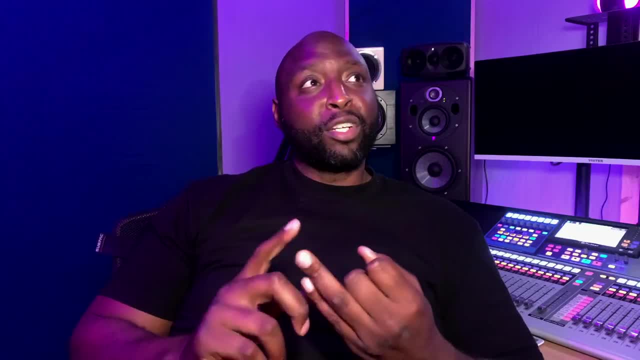 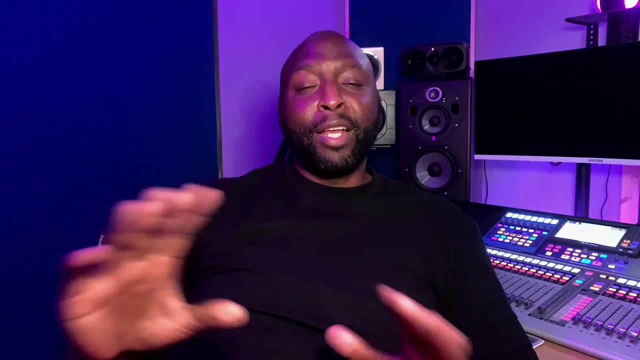 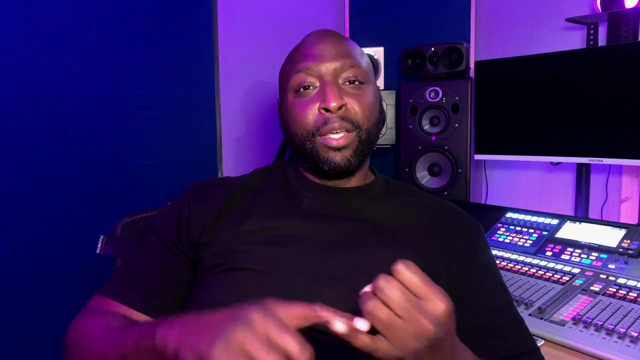 a compressor or like an EQ. um, those are. those are going to be your two main things that you're going to be using is compression EQ. I mean, obviously you can do effects, but right now, let's just talk about this, the pure basics of what you are going to be learning about, which is EQing, and 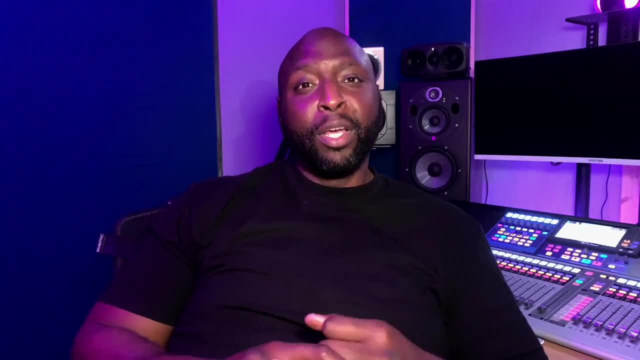 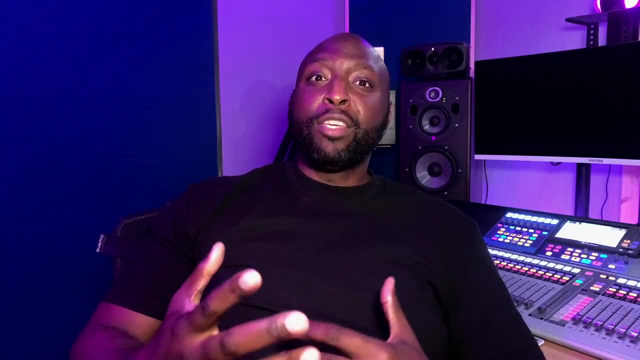 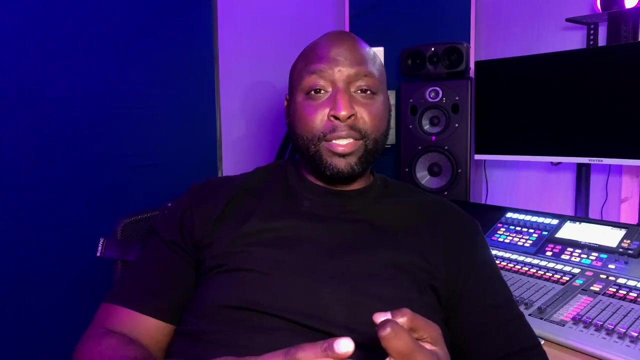 which is compression and knowing when to EQ and when not to EQ, knowing when to not compress too hard and knowing when you need to compress more. so EQ is tonal balance. so think about when you're in your car and you have the bass, treble and the mids- usually those three basic. 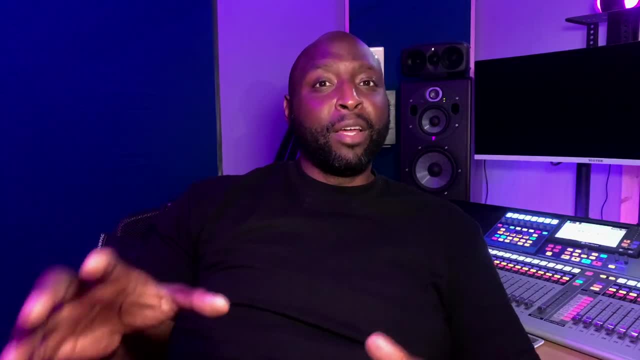 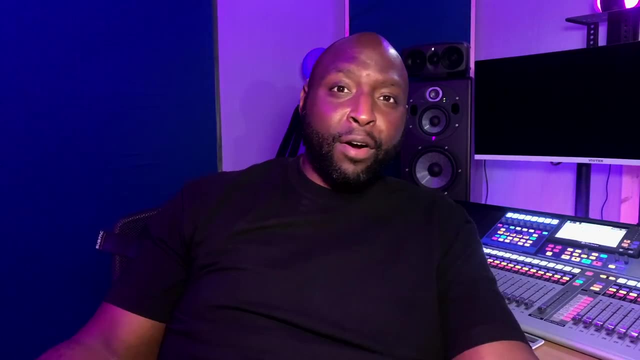 ones are like on the very basic ones, then you'll still. you'll have other car audio systems that might have a little bit more control, but for the most part that's what they're breaking it up into. so say, for instance, you get in your car and you are listening to a 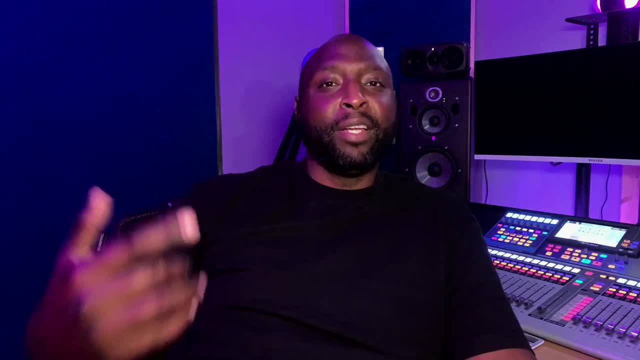 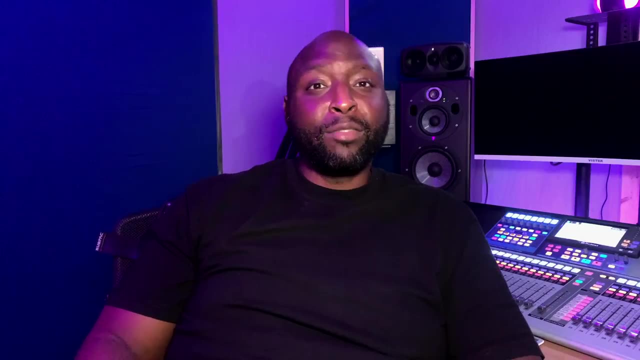 song and then, like you feel like man, this song doesn't have enough bass. I don't feel it enough, so you're gonna go to the bass and you're gonna turn the bass up, or it might sound a little too bright, it might hurt my ear, so I'll go to the treble. let me turn the treble down just a little. 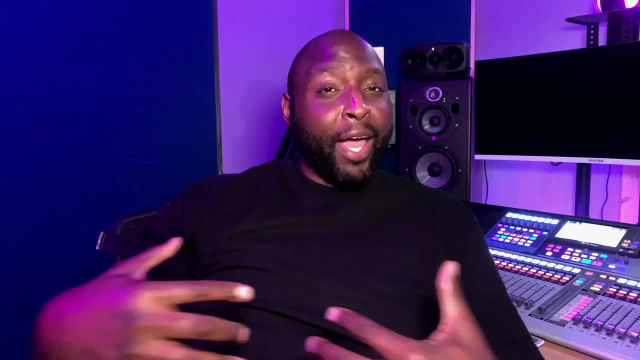 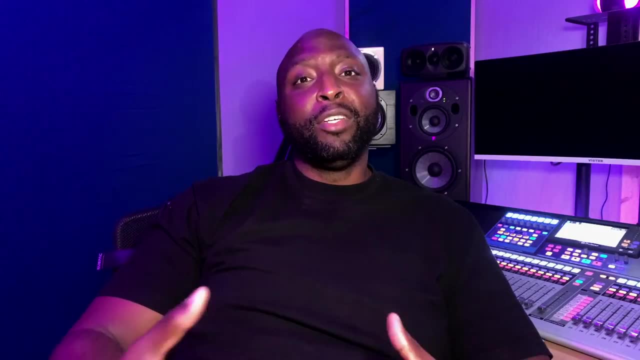 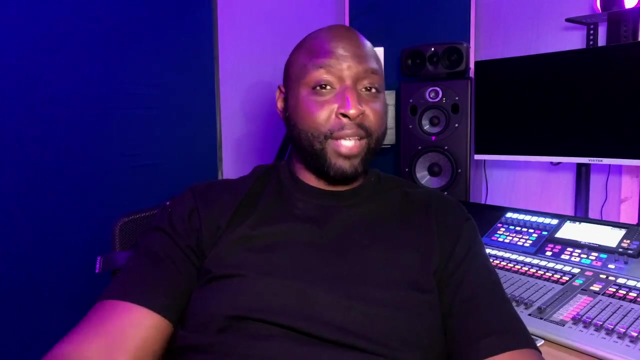 bit. um, that's literally what you're doing as a engineer. okay, you're manipulating the sound so that it sounds good. now, the reason why you're able to do this is because you've heard numerous amounts of music and you can tell when something doesn't sound right, just like when you 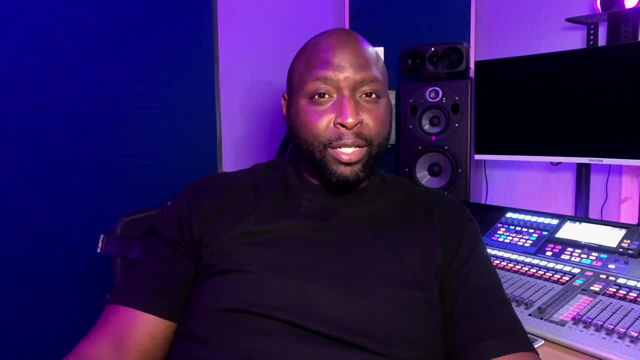 get in your car and if something doesn't sound right to you, you'll know it pretty quickly. because you've been driving in your car for a long period of time, you know what those speakers sound like and you know when something doesn't sound good in there and it's the same thing. that's what. 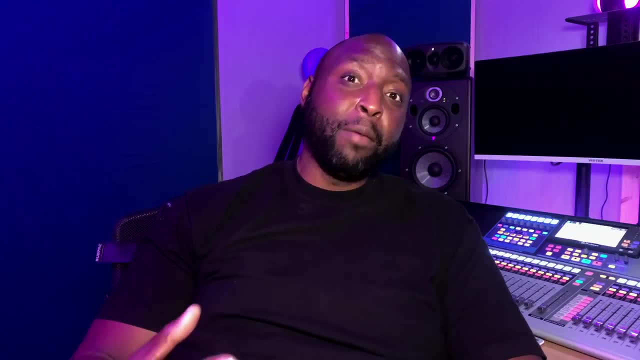 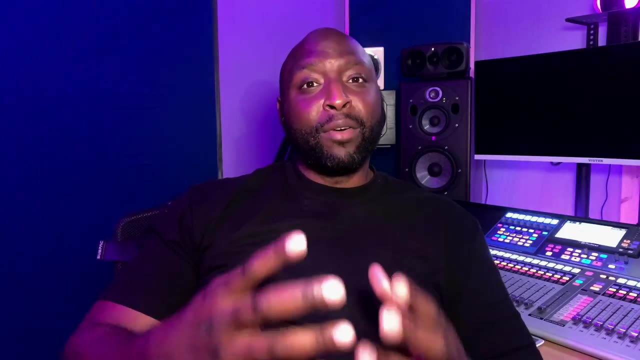 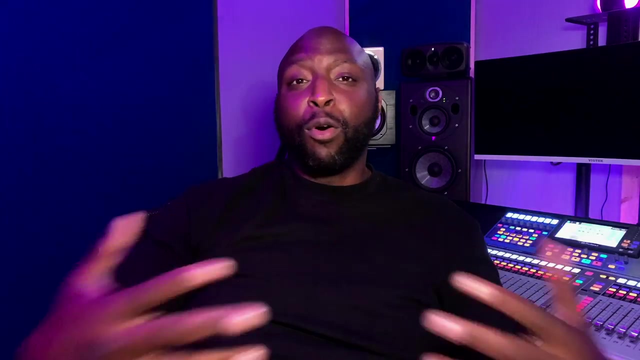 I want you to start thinking about when it comes to being an audio engineer. now. you might be an artist and you want to record yourself and you might want to get your music to sound good. now you have one of two choices. you can be a recording artist who can, who simply just records themselves, and then 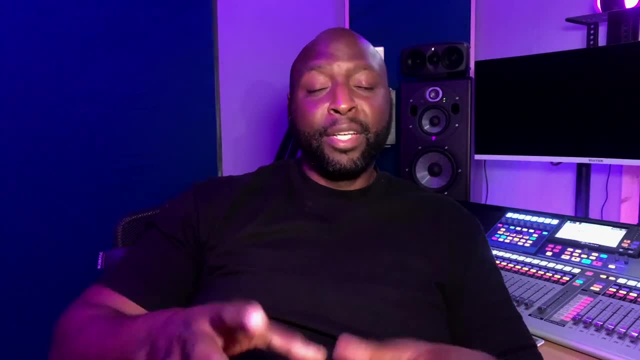 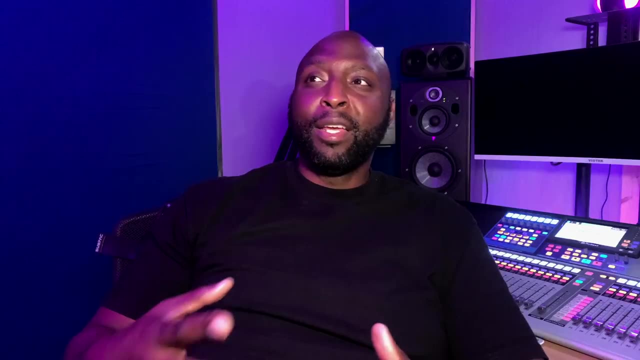 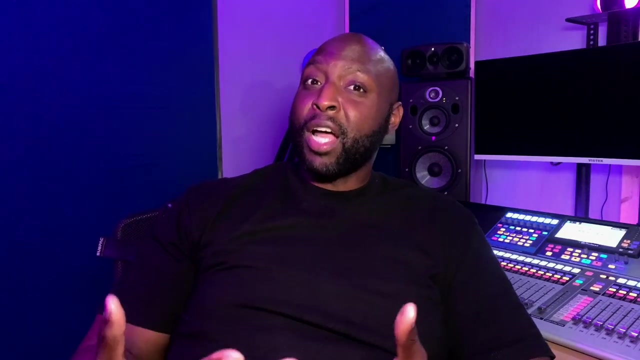 when they're done recording themselves, they send that session to an audio engineer and then the engineer makes the music sound amazing. when I meet women and on these dating sites and stuff, and then here I was actually shocked how many people didn't know exactly what that was. so my favorite answer: 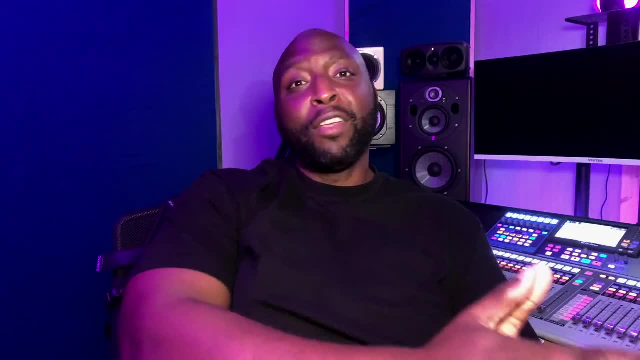 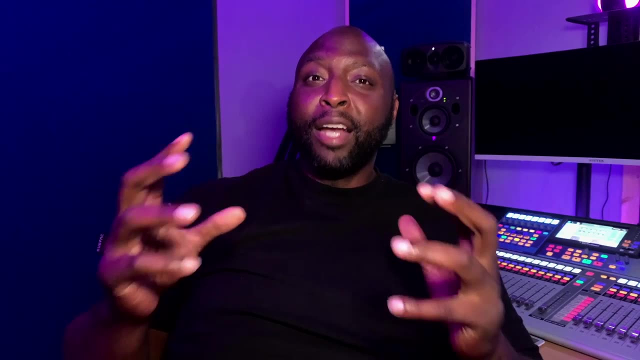 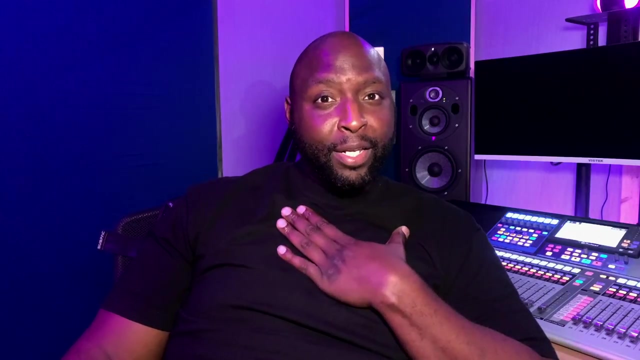 to always give is whoever your favorite artist is, whether it's Beyonce, Michael Jackson. if they didn't have a really good audio engineer, they would not sound good on the radio. the audio engineer, in my opinion, is more important than the producer and the artist, because the audio 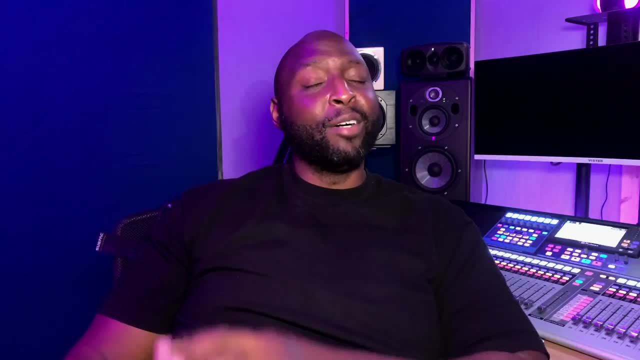 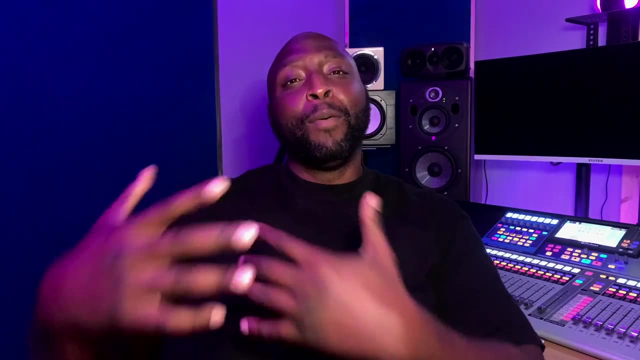 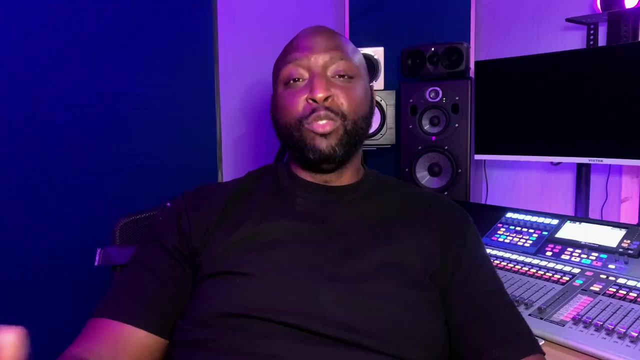 engineer is the person who makes sure everything sounds great. now you have a mastering engineer and that's that's. that's just going. that's going further. but the point is, the audio engineer is very important to the success of any project that you've ever heard. they're the ones who made it to 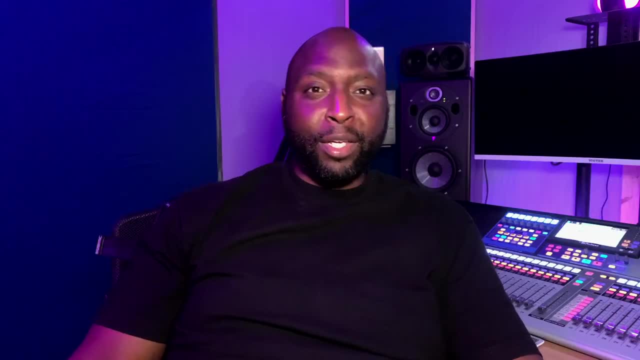 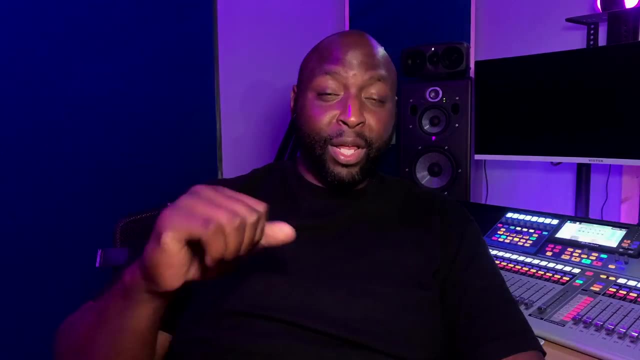 where, when you heard it, you had an emotion. you felt something. something made you cry, something made you happy, something makes you want to dance, something made you want to ride in your car too. like all of that is technique that audio engineers have. then give you an experience. 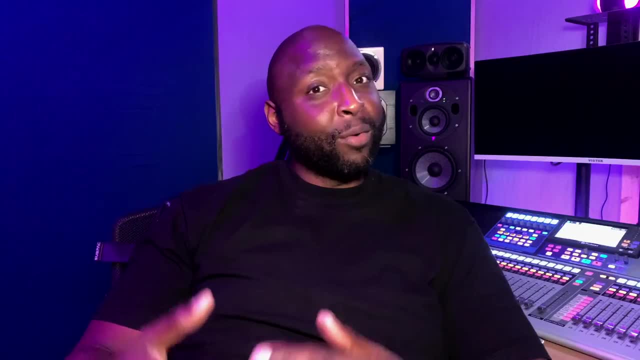 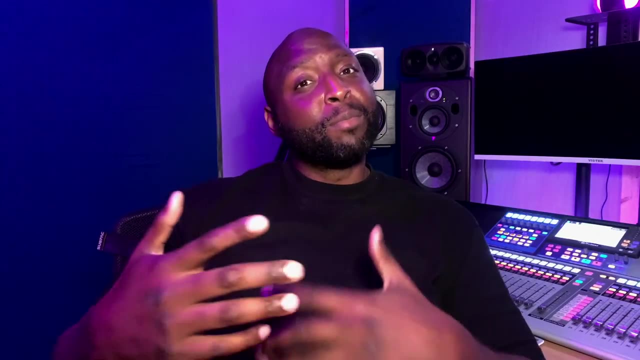 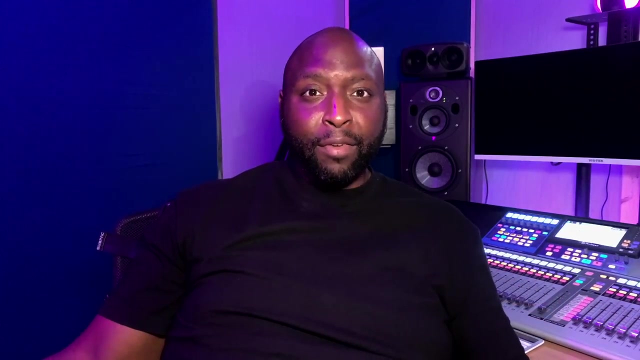 and that's what an audio engineer does. so you might want to really think: is that something as an artist that I want to do, or do I just want to focus more on the artistry and send it to somebody else who does the audio engineering as a living? that's pretty much as simple and as basic. 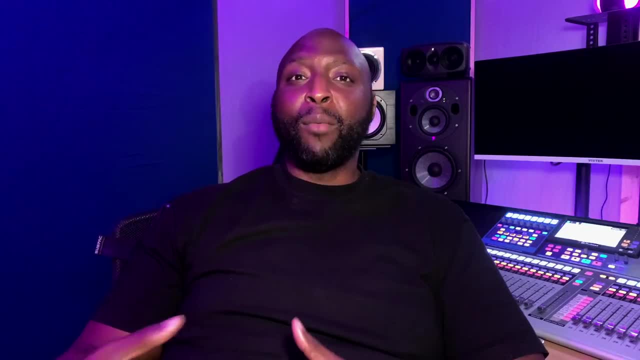 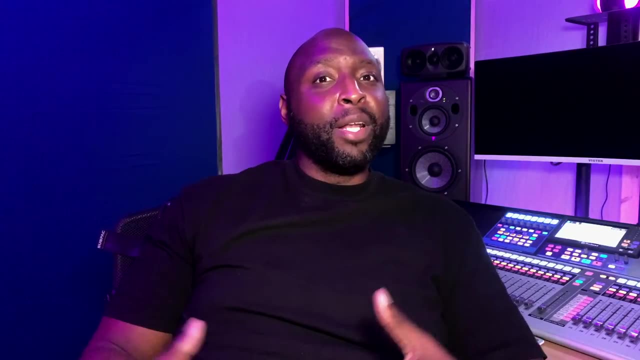 some techniques. so if you are deciding that, hey, you know what i want to record myself, but i don't have money to pay an audio engineer, but i do just want to make it sound decent enough to put it up on soundcloud, well then you might want to subscribe to this channel. i'm just telling you right now. 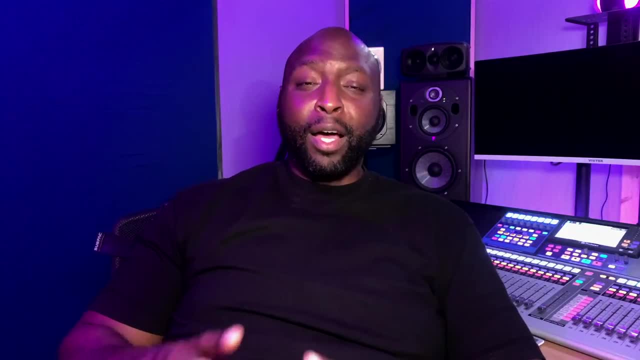 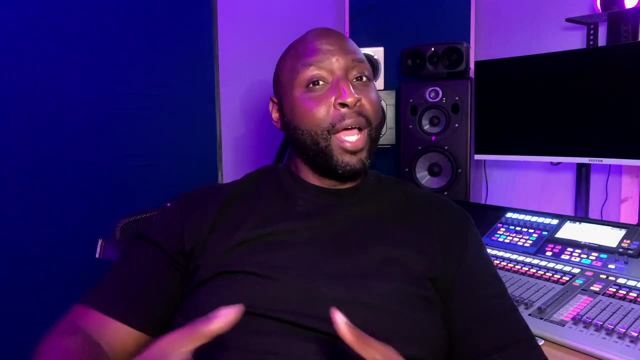 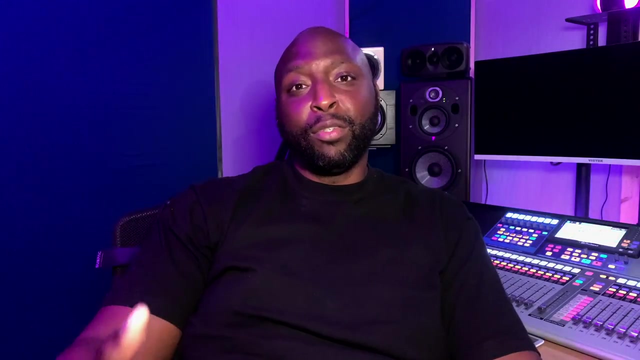 because i'm going to start giving you basic things that you can do um to make your music sound great, so they're not going to be too advanced. i will try to make it as simple as possible and when i you know i show these things, i'll tell you why i'm doing it, so that in any situation that you 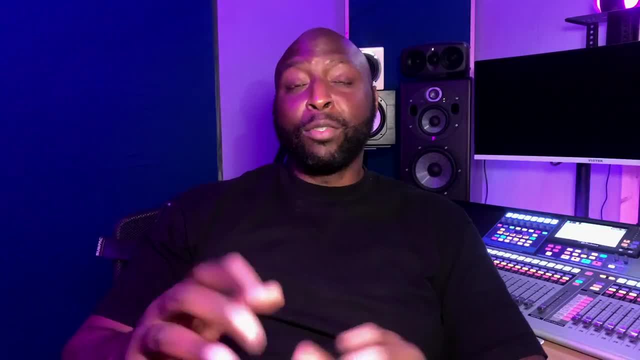 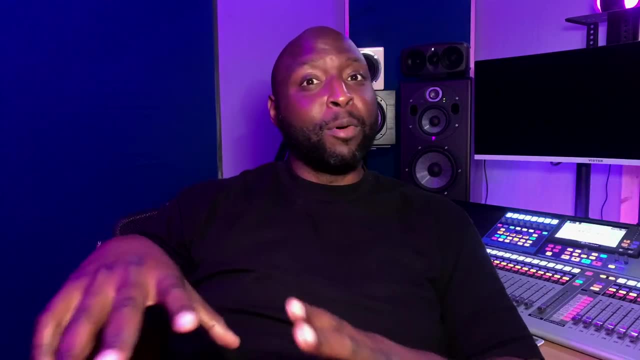 were presented with, you'll be able to make the right decisions. i'm going to go to the next video. as a matter of fact, i'm going to start recording the next video right now, so it's possible that this video might be coming out in the next few days. so hit that subscribe button and thumbs it. 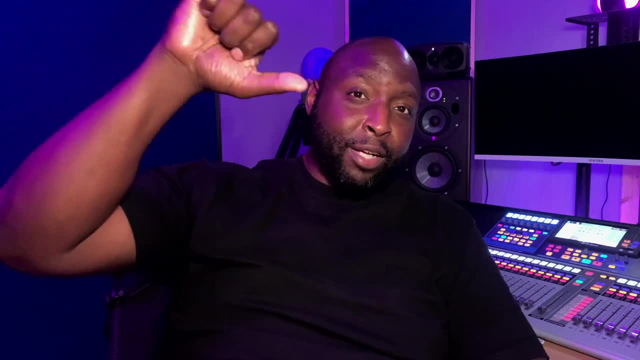 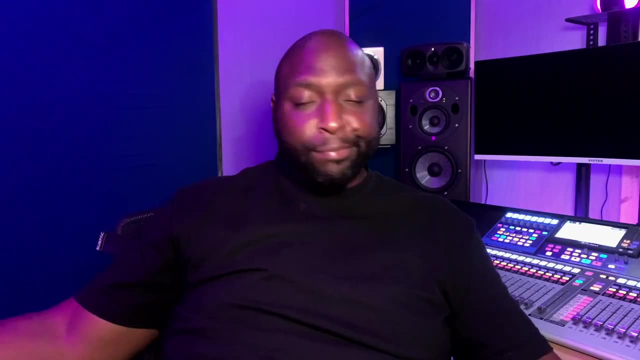 up if it's something that you are interested in, and if it's something that you want to thumbs down, that's great. just tell me why you're thumbs downing the video, because you know, if it's something that i feel like i could probably adjust, i'll do so anyhow, i. 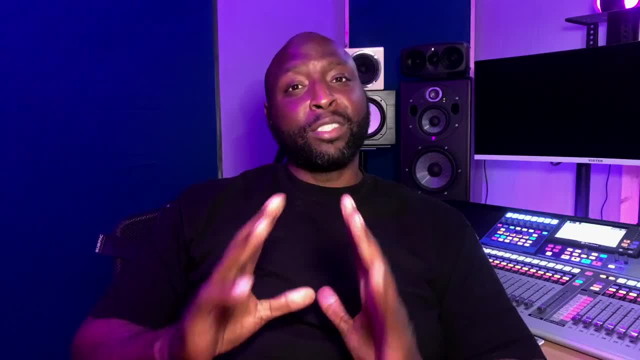 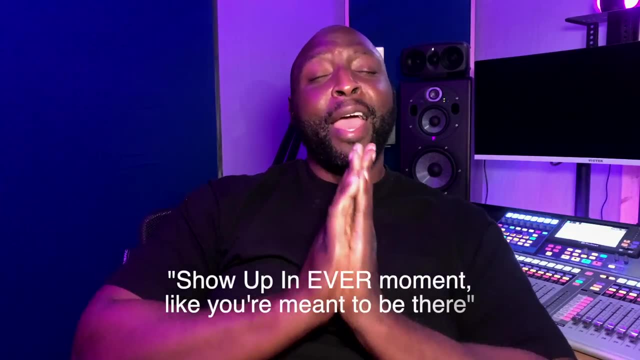 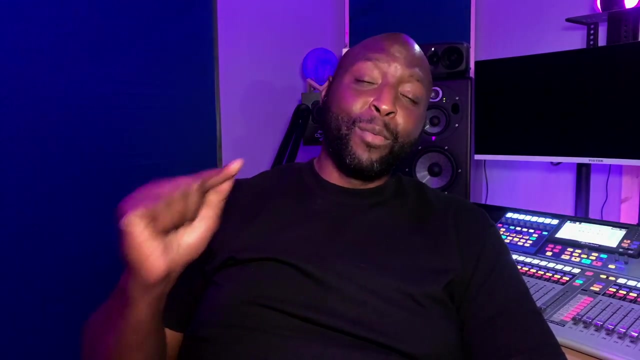 will catch you guys and, oh, before i go, before i go, i actually want to start doing this with every single video, i want to give you guys a quote of the day. so today's quote is going to be show up in every moment, like you're meant to be there and i. that is. that is key if you're, if you're out here. 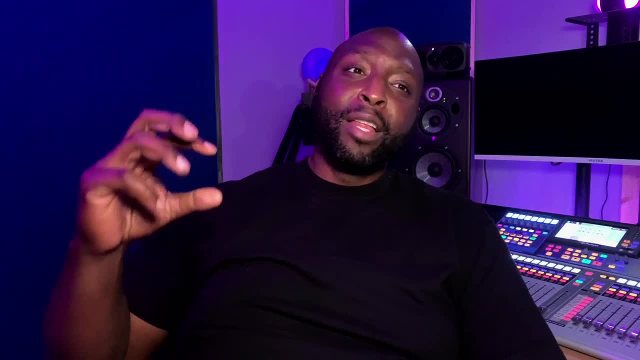 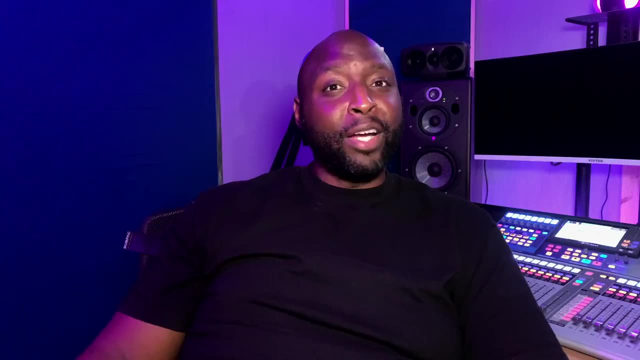 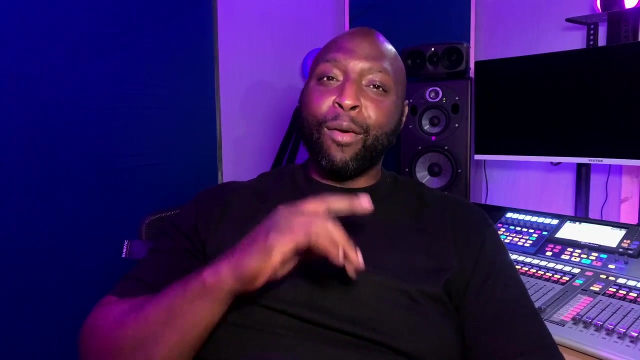 trying to be an audio engineer. you need to know that, no matter what, you're going to be the most important person in the room full of artists, because if they know you are an audio engineer and you're good at what you do, they will come because they need you anyhow. all right, i really